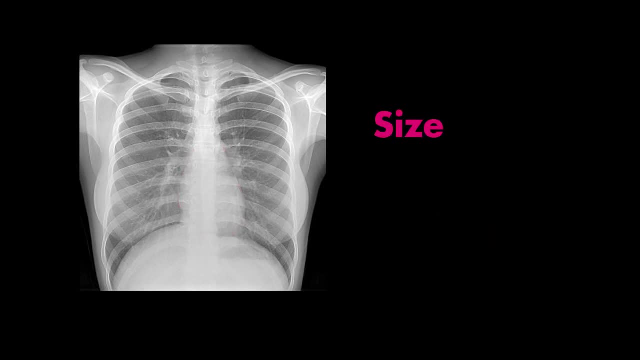 size of the heart and the position of the heart. In one of the first videos we briefly talked about the cardiac silhouette. Depending on what type of x-ray view you are looking at, the cardiac silhouette should be no larger than half the size of the patient's thoracic cavity. 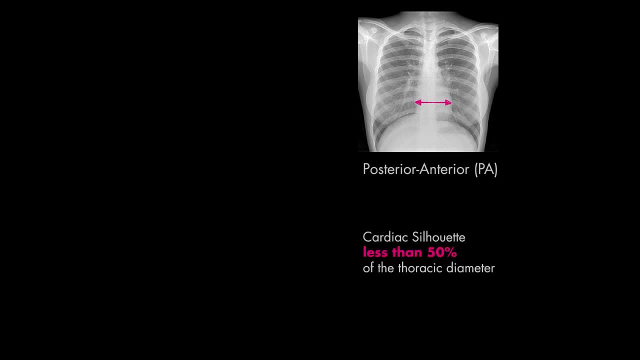 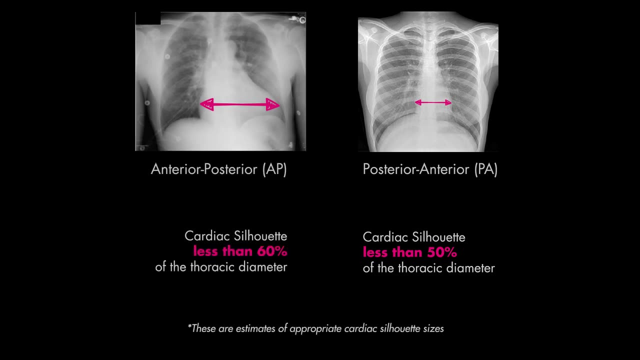 More specifically, on a PA film the cardiac silhouette should be less than 50% of the chest diameter and on an AP film we will accept a cardiac silhouette less than 60%. Remember that on an AP film that the heart will seem artifactually larger because of 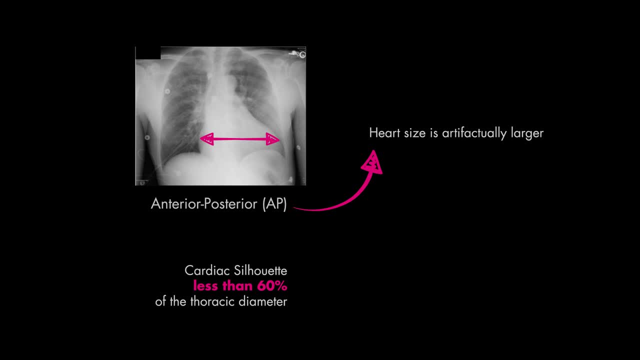 the way the film was shot. If you haven't already seen the video on chest x-ray positioning and views, please check it out by clicking the link for part 4 of this video series in the description below. So heart sizes larger than what we just mentioned can imply many things, but by far the most. 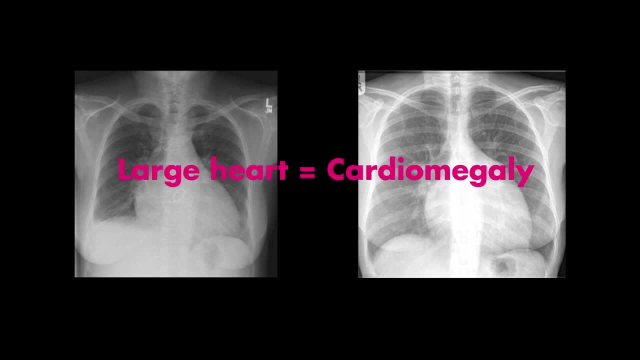 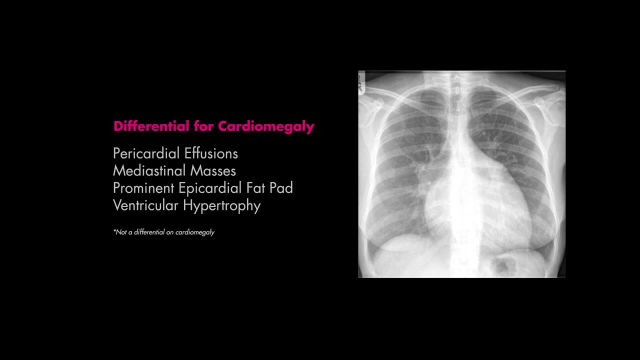 common is cardiomegaly or an enlarged heart. The reason for this also has a long differential, but you should start thinking of things like pericardial effusions, mediastinal masses or a prominent epicardial fat pad. Over time. patients with long-standing hypertension can also result in left ventricular hypertrophy, leading to a larger heart. Enlarged heart sizes can also be exaggerated. if your chest x-ray was obtained during expiration, In this case, the thoracic diameter would be smaller in comparison to the heart, which 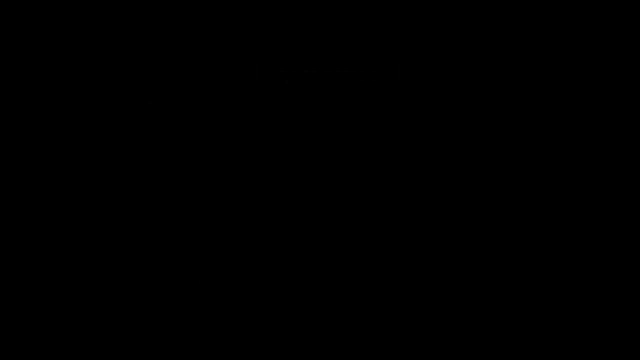 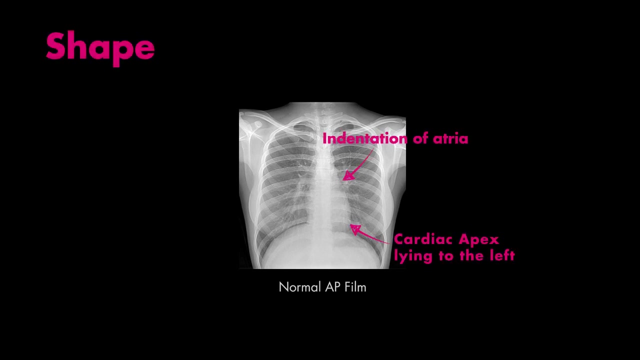 would seem relatively larger. Other considerations when assessing the cardiac silhouette include looking at the heart shape, which would look like this: In the cases of very severe cardiomegaly, the heart may seem more round, like you see here. In the cases of very severe cardiomegaly, the heart may seem more round, like you see here. 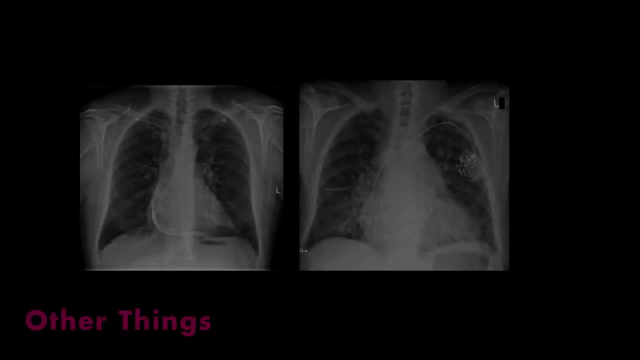 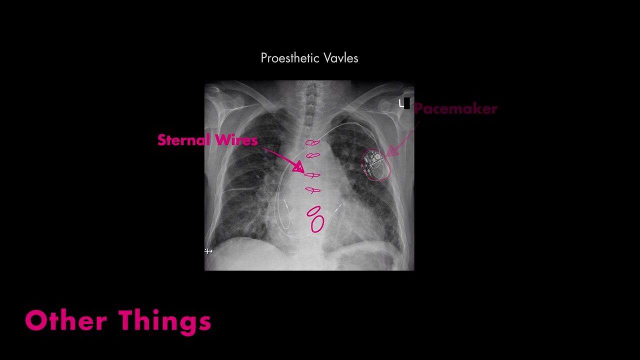 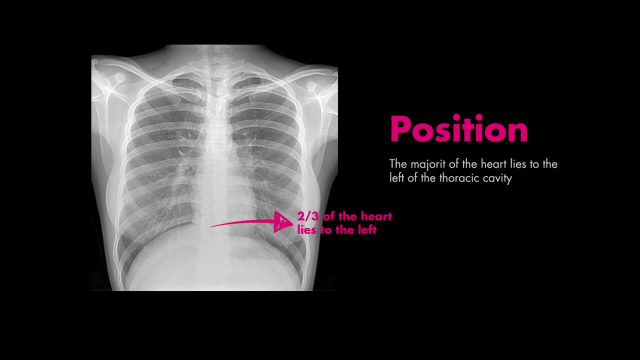 Other things you may notice include calcifications and prosthetic valves. Other things you may notice include calcifications and prosthetic valves. Lastly, make note of the heart position. Normally two-thirds of the heart lies to the left of the thoracic cavity. on chest x-ray. 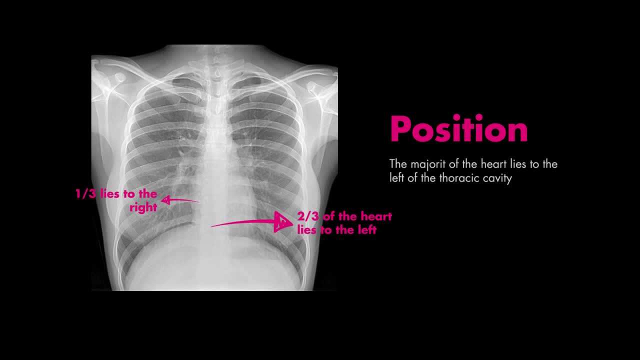 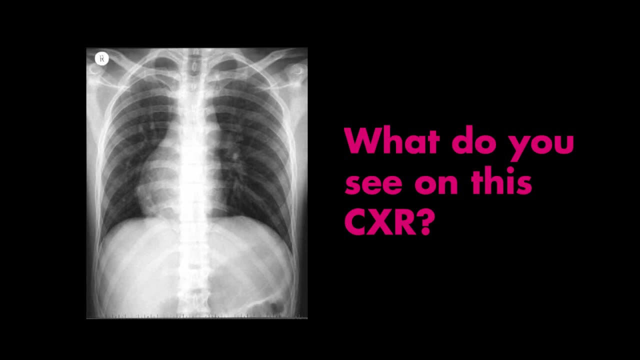 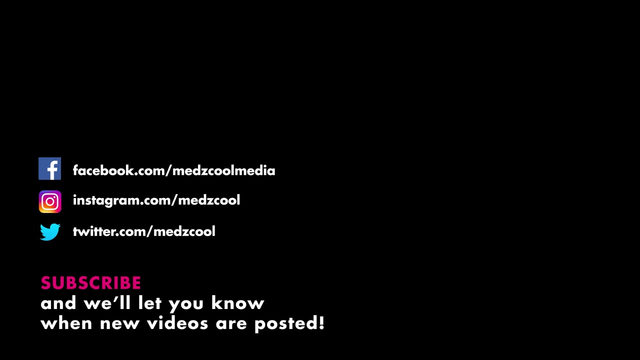 and roughly one-third of the heart lies to the right. I'll leave you with this last x-ray. What do you notice about this chest x-ray and the cardiac silhouette? Leave your thoughts in the comments. If you haven't already, make sure to subscribe to this channel to get updates on when we 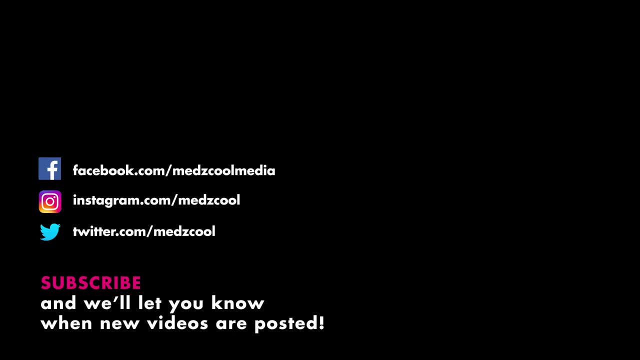 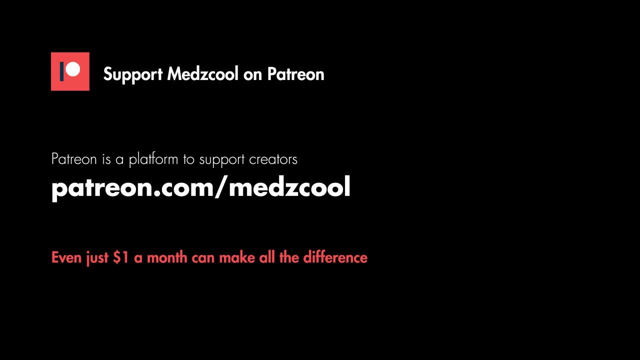 release our latest videos and don't forget to follow med school on social media. If you're feeling real generous, visit our Patreon page and make a pledge to help us create more awesome videos.